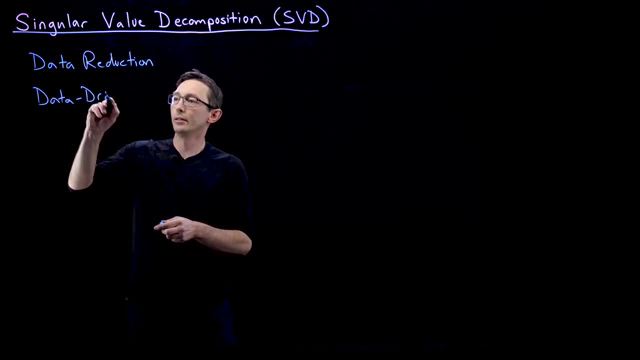 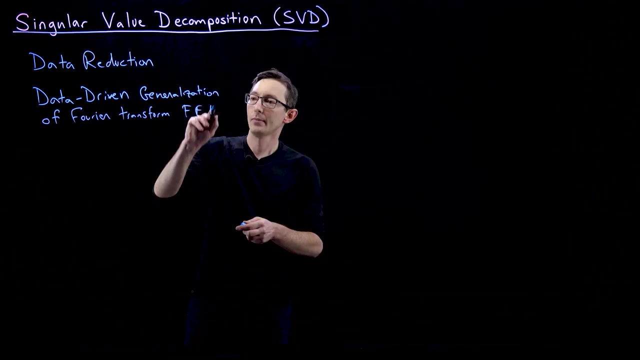 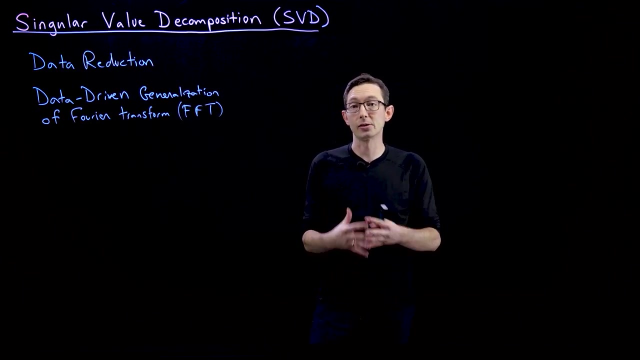 transform, So data-driven generalization of the Fourier transform And I'm just gonna say the FFT. So the FFT is one of the most useful transformations in all of mathematics, based on sine and cosine expansions to approximate functions. There's also Bessel's functions, Aries functions, spherical harmonics And this. 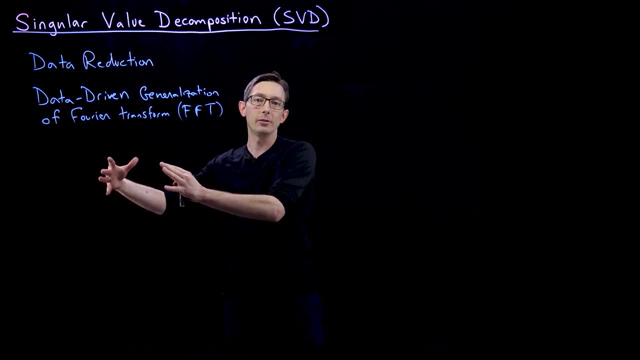 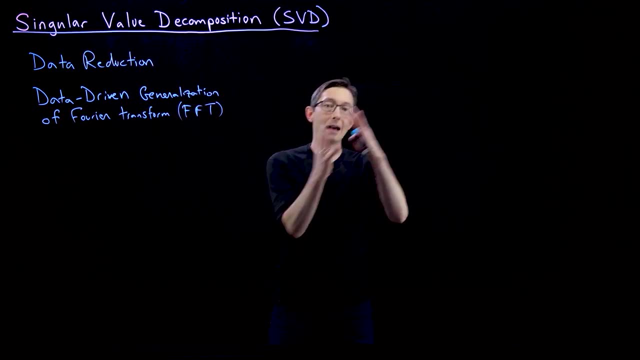 was the technique of the last generation of computational science and engineering, was to use these mathematical modes, these mathematical transformations, to map a system of interest into some new coordinate system where it would become simple. But in many systems of interest today, like let's say, 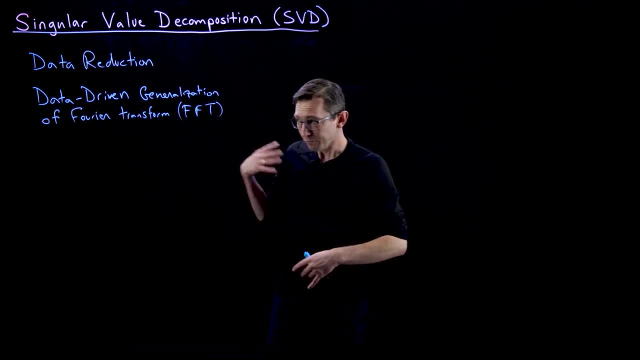 I have a turbulent flow of over a bowing wing. there isn't an easy off-the-shelf mathematical transformation or set of basis modes that describes that behavior, And so what the SVD- the singular value decomposition- is going to allow us to do is to tailor a 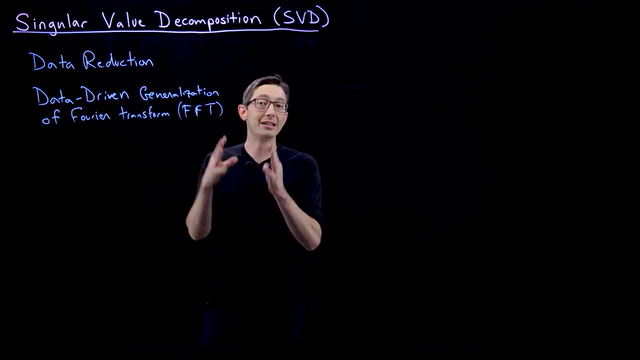 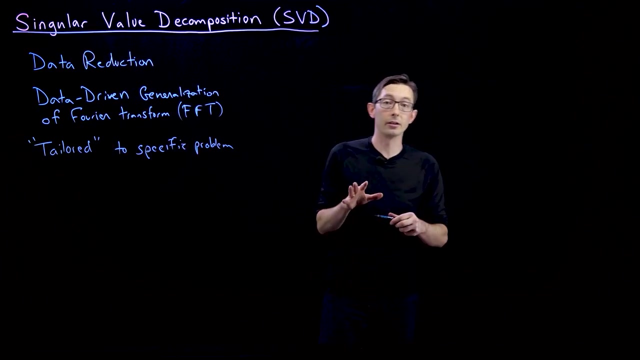 coordinate system or a transformation based on the data that we have. So I think of these as tailored to the specific problem. Okay, so they have a lot of features in common with the Fourier Transformers- we're going to learn throughout this video sequence- but it's tailored to. 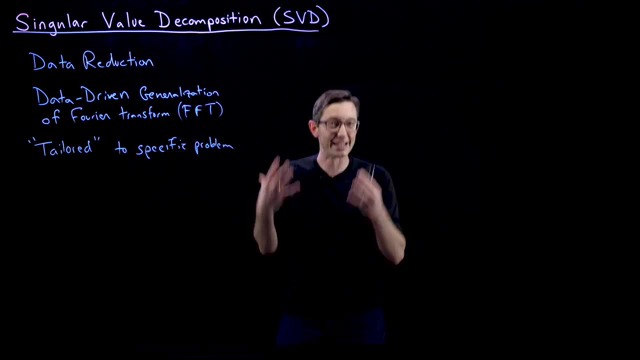 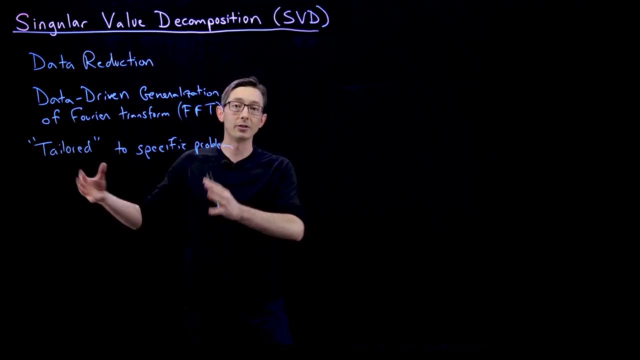 specific problem that you're interested in to the specific data that you have access to. So in the next lecture I'm gonna go through actually defining a data matrix, how you compute the SVD and what it means. Here I just want to tell you kind of how you can use it. 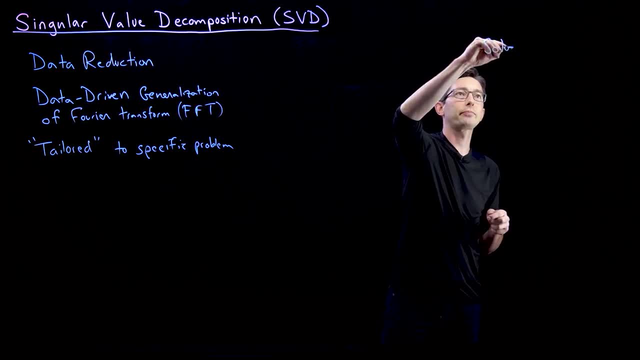 So one thing you can do is you can use it to solve matrix system of equations A, X, E, D, I and V, And this actually works for anything that you're interested in, because you're just, you're just, you're interested. so once you understand that fifteen stands for You as长, FVD and 2,. 1, and 2, this doesn't mean you're not kinetic, but it can be end of the system, orilight instead. 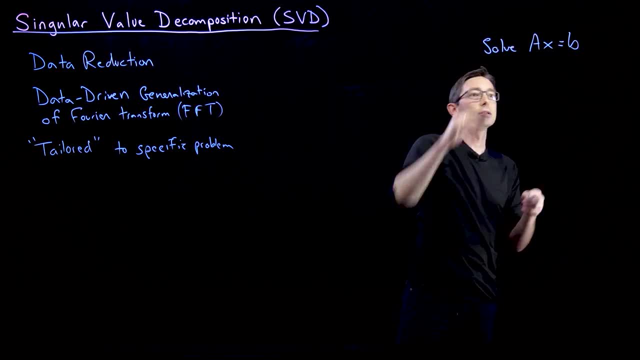 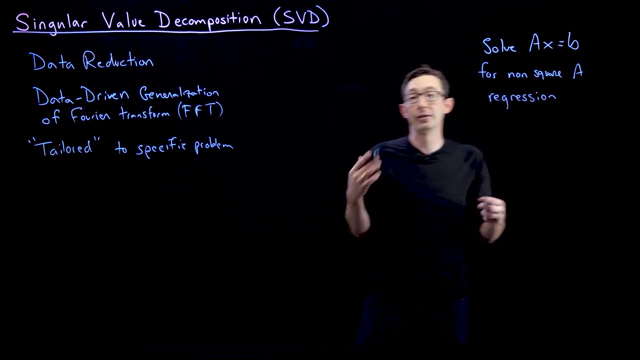 system of equations AX equals to B, so linear systems of equations for non-square A matrices, And we're going to use this in particular for linear regression models and for many other things. So if I have data, let's say health data, for a bunch of patients and I want 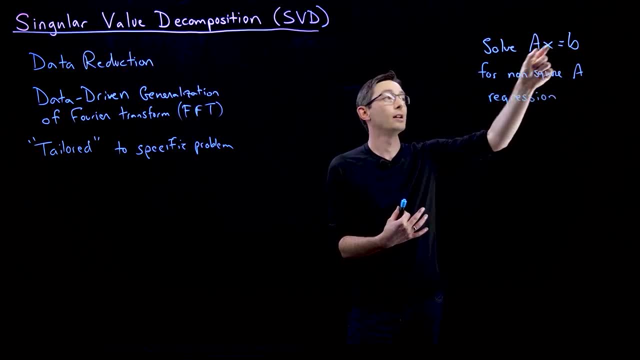 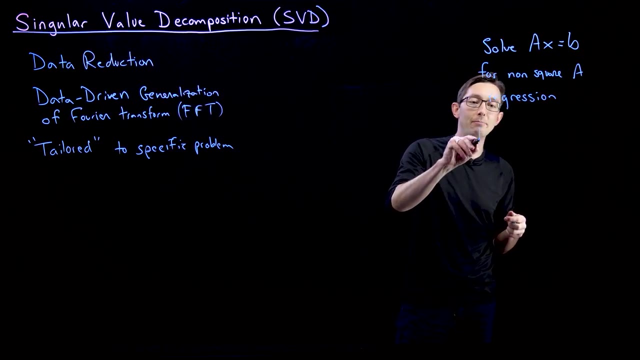 to build a model of how different risk factors map to some disease. I can build the best fit model X, given data A and B, using least squares. linear regression, Again built on the singular value decomposition. I can also use this as the basis for the principal component. 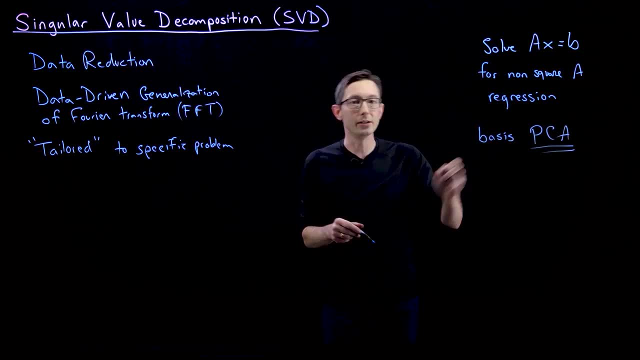 analysis, PCA- which is one of the most widely used techniques in all of statistics for taking high dimensional data and trying to understand it in terms of its dominant patterns or correlations. So that's a key word we're going to talk a lot about as we go along. 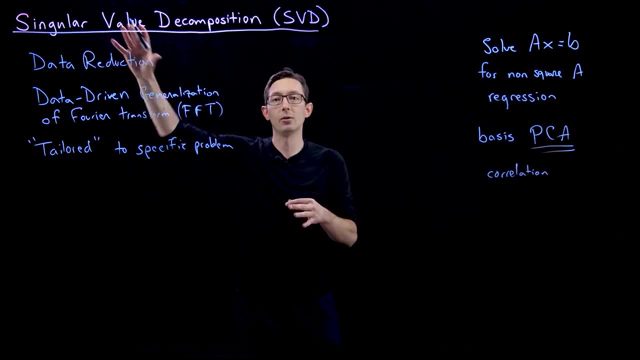 So we're going to talk a lot about the singular value decomposition and we're going to talk a lot about the key features that are involved in this. So the singular value decomposition is going to take high dimensional data and distill it down into the key features. 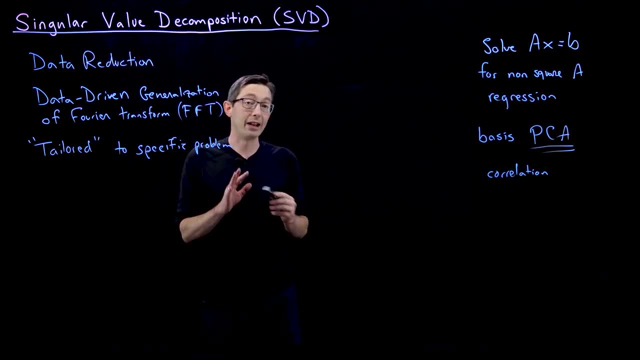 the key correlations in that data that you can then use to interpret and understand and model that data. It really is used everywhere. It's used in Facebook, Google, Microsoft, So, for example, it's used in the Google page rank algorithm. It's used in a lot of websites. in an order: 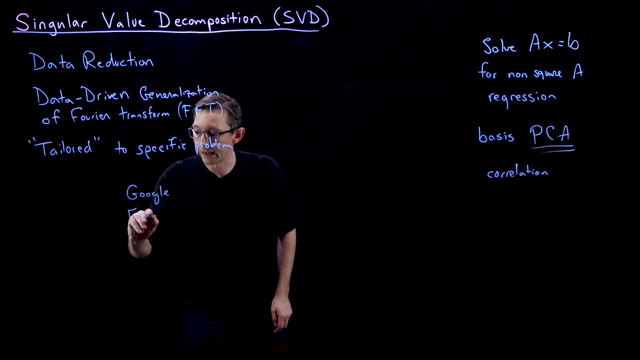 It's using an SVD for that singular value decomposition. It's the basis of many, many facial recognition algorithms to tell which person is who from an image, So you could again build these singular value decomposition representations of human faces. It's also used in recommender systems like Amazon and Netflix. 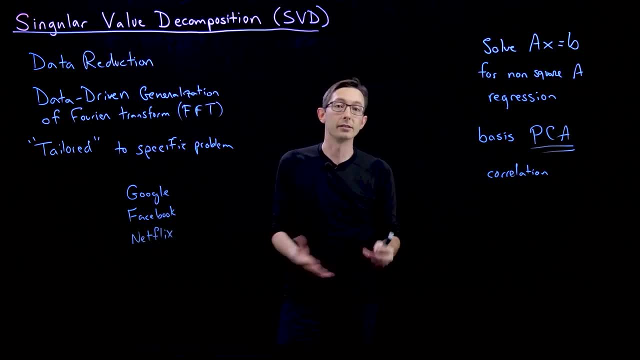 where it will essentially build correlation patterns of what types of people like what types of movies. And this is just a very, very, very brief list of all of the examples of the SVD in industry. So I always like to tell my students that the SVD is one of the most important algorithms. 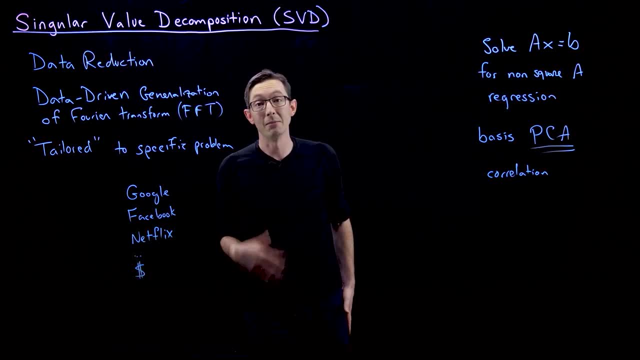 if you want to actually use linear algebra to make money, So very, very useful. Part of the reason it's so widely adopted is because it's based on very, very simple linear algebra- simple and interpretable Linear algebra, which means that you can use it really.